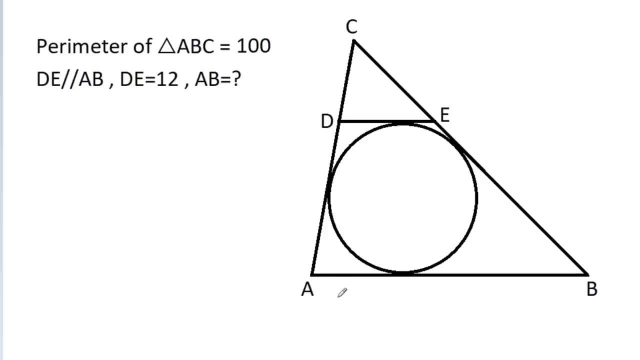 In this video we have been given that perimeter of triangle ABC is 100 and DE is parallel to AB and DE is 12, then we have to find AB. So suppose this point is P, this point is Q, this point is R and this point is S. Then in any circle, from any point, P, 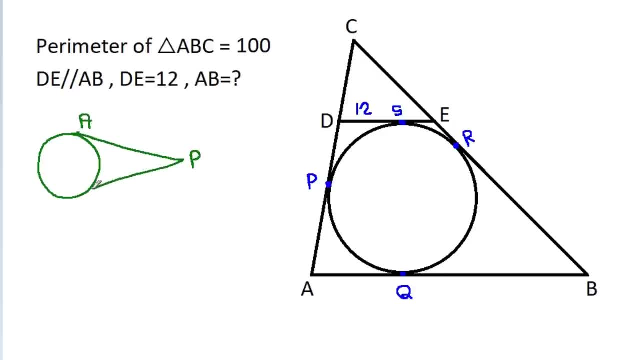 if PA and PB are tangent, then PA it will be equal to PB. So here, from point A, AP it will be equal to AQ. Suppose A, AP is A and AQ is A, And from point B, BQ. 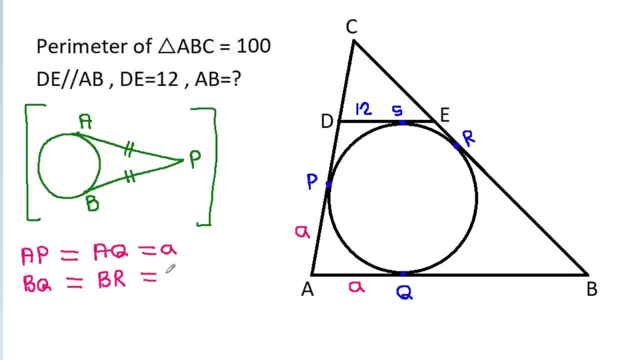 it will be equal to BR. Suppose B, BQ is B and BR is B And from point C, CR it will be equal to CP. And suppose CE is C and ER is D, Then CR it will be equal to. 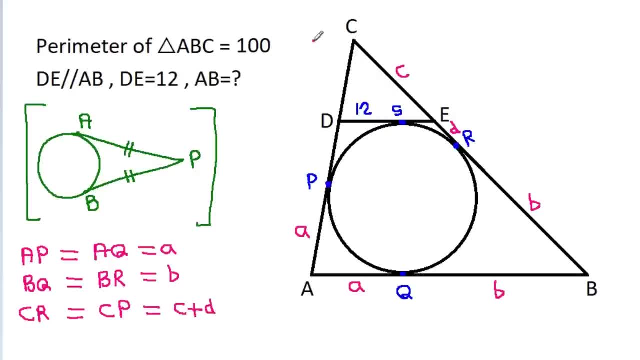 C plus D, So CP it will be also C plus D, And from point E, ES it will be equal to ER And ER is D, So ES it will be D, And we have DE is 12.. 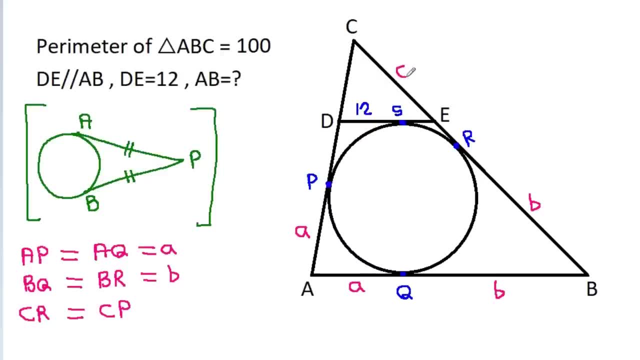 And suppose CE is CE And ER is D, Then CR it will be equal to C plus D, So CP it will be also C plus D, And from point E it will be also C plus D, And from point E ES it will be equal to ER and ER is D. 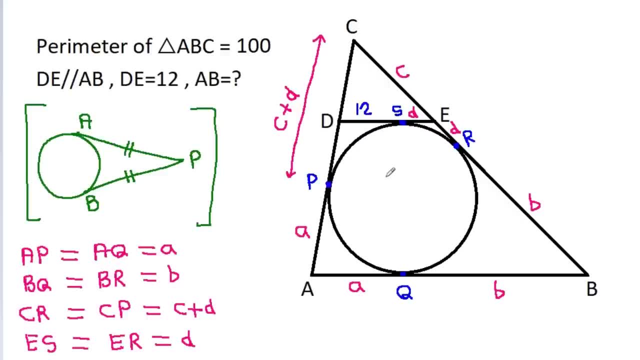 So ES it will be D And we have DE is 12.. So DS it will be 12 minus D And from point D, DP it will be equal to DS And DS is 12 minus D. 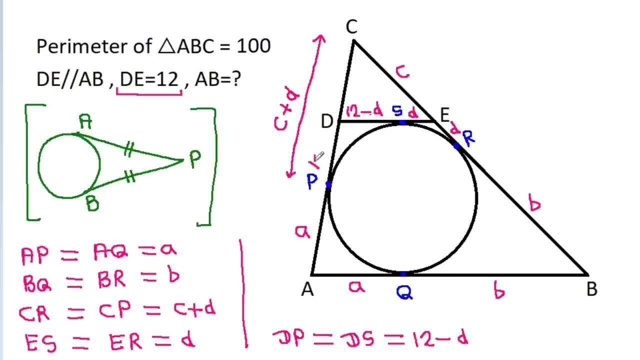 So DP it will be 12 minus D, And CD it will be equal to CP minus DP, And CP is C plus D minus DP, is 12 minus D, And it is C plus D minus 12 plus D And it is C plus 2D minus 12.. 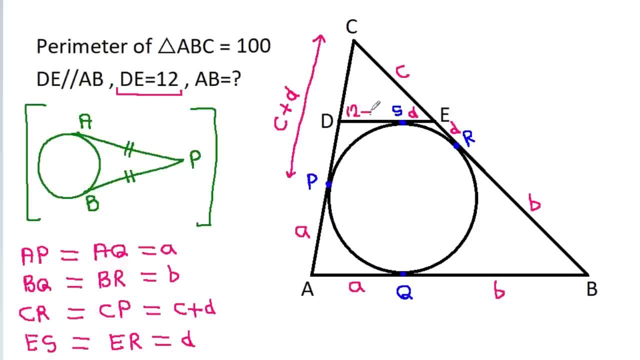 So DS it will be 12 minus D, And from point D, DP it will be equal to DS, And DS is 12 minus D, So DP it will be 12 minus D And CD it will be equal to. 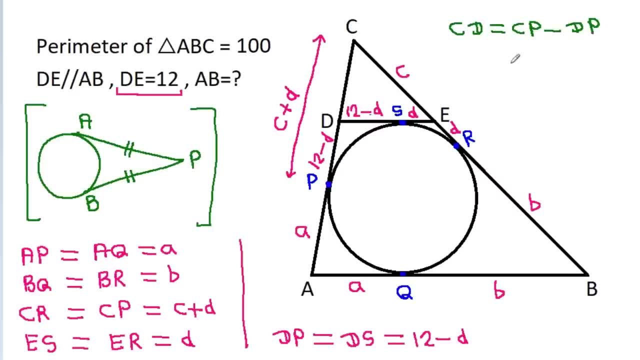 CP minus DP And CP is C plus D minus DP, is 12 minus D, And it is C plus D minus 12 plus D And it is C plus 2D minus 12.. So CD, it is C plus 2D. 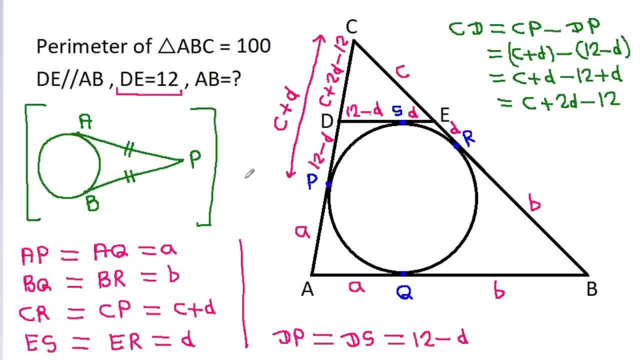 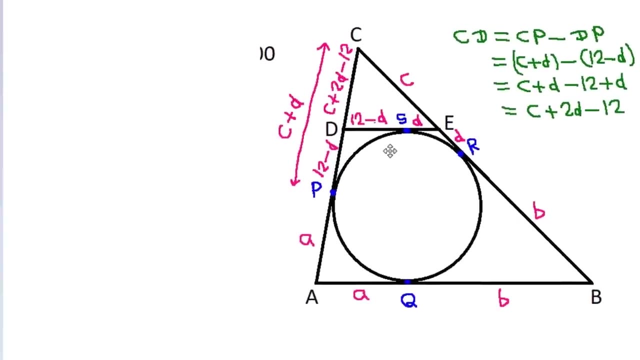 minus 12.. And now we have given that DE is parallel to AB, So in triangle ABC it is DE And DE is parallel to AB. That means these two angles will be equal And also these two angles will be equal. 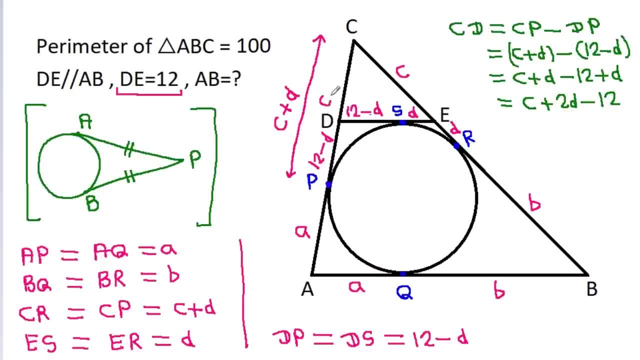 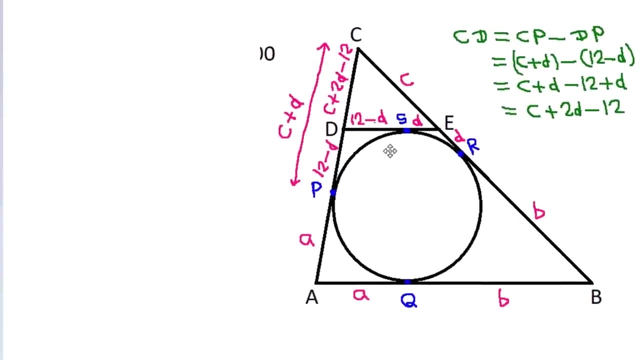 So CD, it is C plus 2D minus 12.. And Now we have given that DE is parallel to AB. So in triangle ABC it is DE And DE is parallel to AB. That means these two angles will be equal. 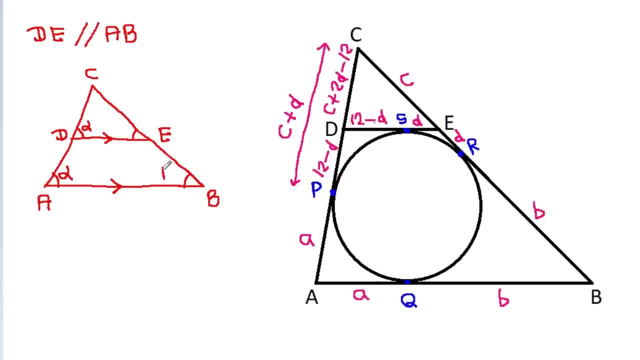 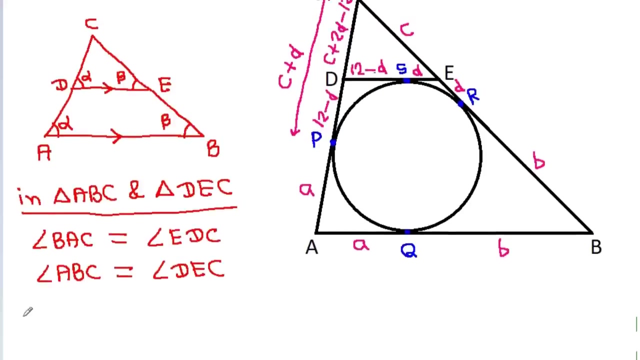 And also these two angles will be equal. So in triangle ABC and triangle DEC, angle BAC it is equal to angle EDC And angle ABC it is equal to angle DEC And angle ABC it is equal to angle DEC. 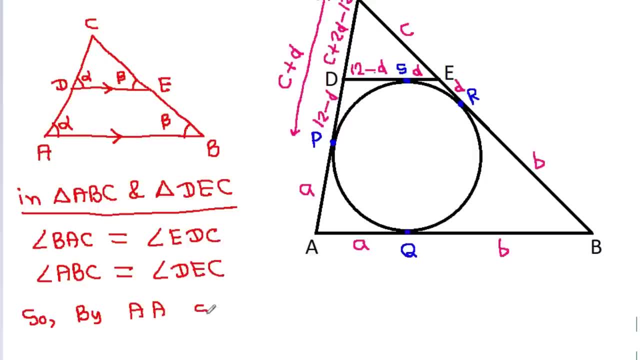 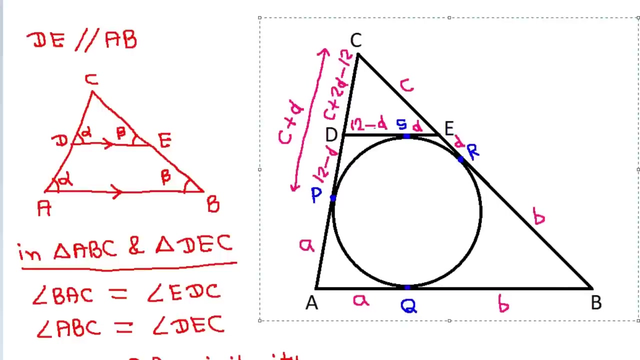 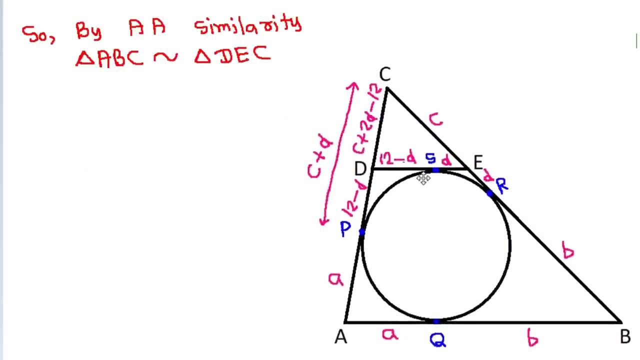 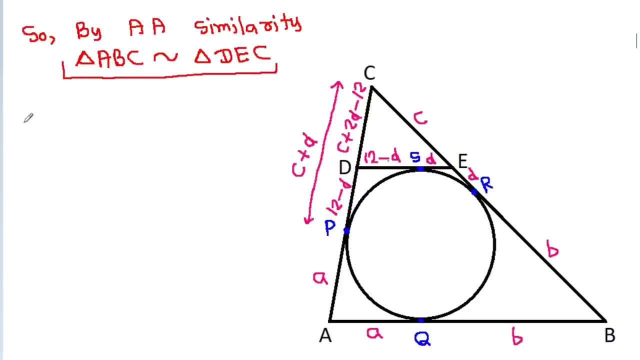 So by angle angle similarity- triangle ABC: it will be similar to triangle DEC. So by angle angle similarity- triangle ABC- it will be similar to angle DEC. And These two triangles are similar. That means perimeter Of ABC. 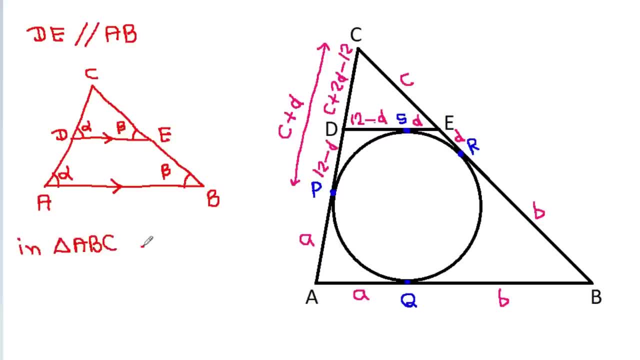 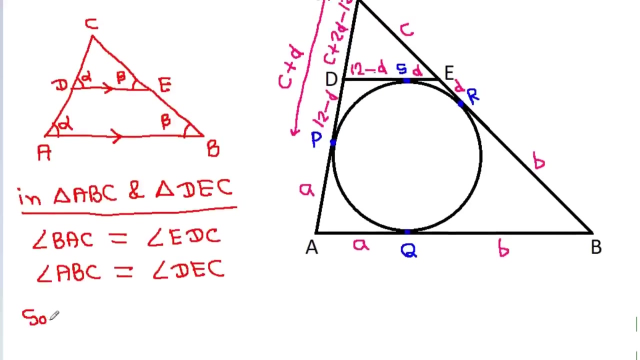 So in triangle ABC and triangle DEC, angle BAC it is equal to angle DEC And angle ABC it is equal to angle DEC. So by angle angle similarity, triangle ABC it will be similar to angle DEC. 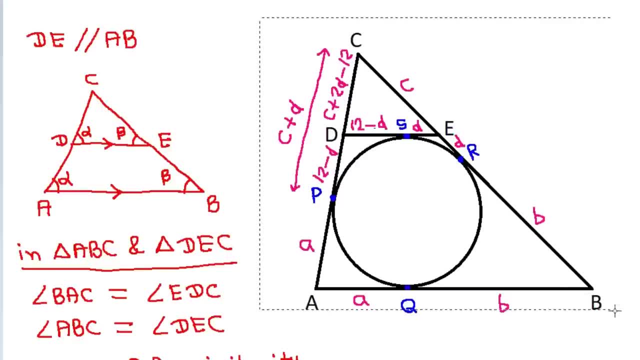 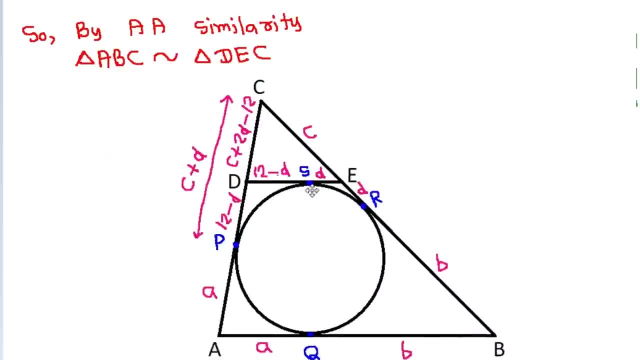 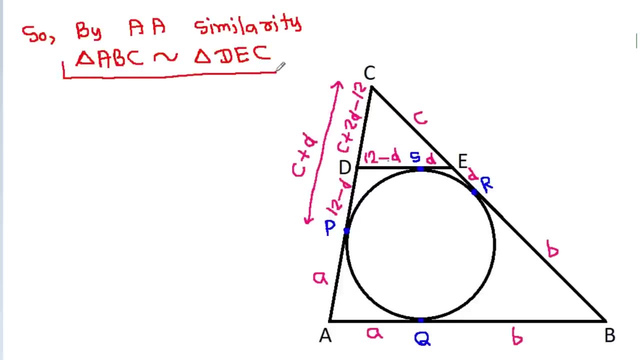 And these two triangles are similar. That means perimeter of AB, of DEC. by perimeter of DEC it will be equal to AB by DE And perimeter of ABC it is 100. by perimeter of DEC it will be CD plus DE plus EC It is. 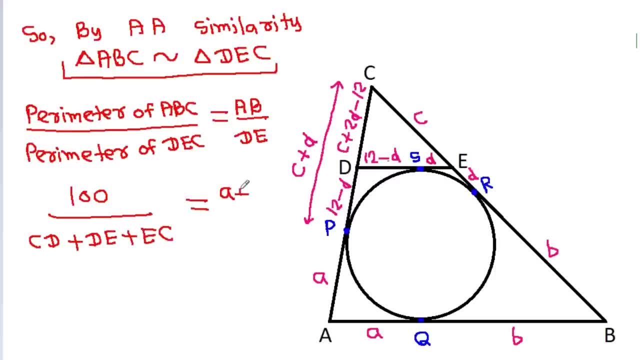 equal to AB, it is A plus B. by DE it is 12 minus D plus D, that will be 12.. And suppose A plus B is equal to X, then it is 100. by CD is C plus 2D minus. 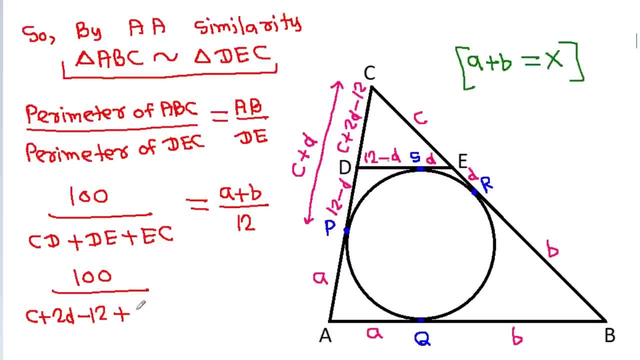 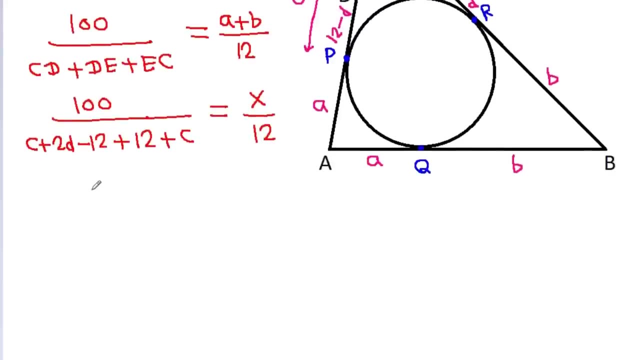 12 plus DE is 12 plus EC is C. It is equal to X by 12. And it is 100 by, and 12 will get cancelled. And C plus C is 2C plus 2D, It is equal to. 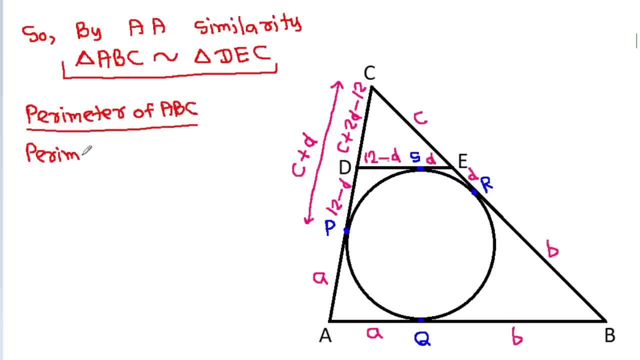 perimeter of DEC it will be equal to AB. by DE and perimeter of ABC, it is 100. by perimeter of DEC it will be CD plus DE plus EC. it is equal to AB. it is A plus B. by DE it is: 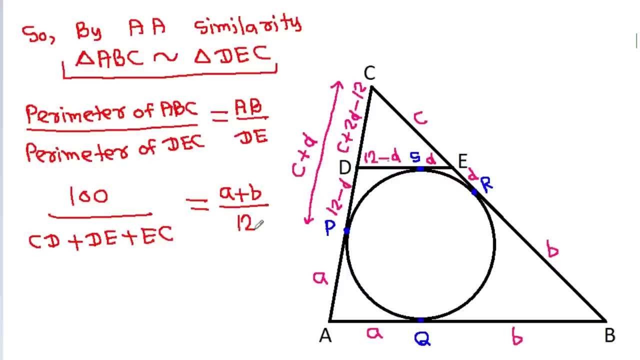 12 minus D plus D, that will be 12.. And Suppose A plus B is equal to X, then it is 100 by CD is C plus 2D minus 2N plus DE is 2N plus EC is C. it is equal to X by 2N. 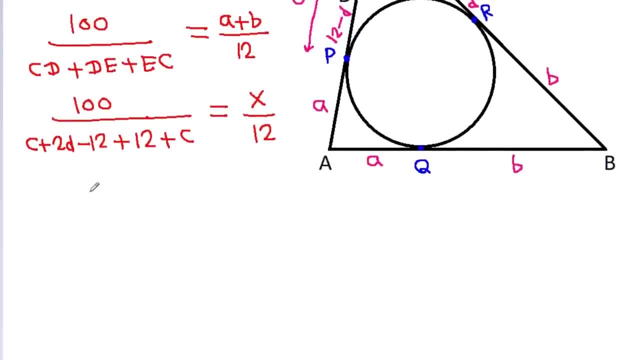 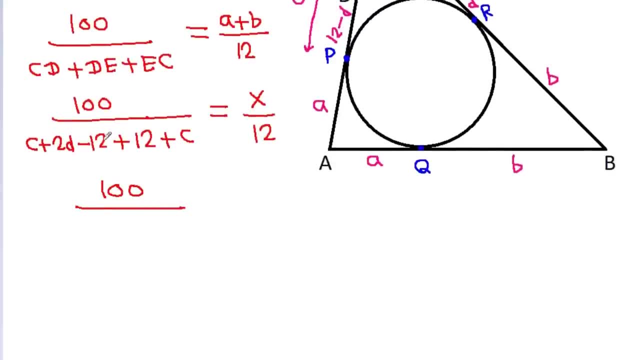 is equal to X by 2N. So let's add e for an example, and here this D, and it is 100 by and 2N windy get cancelled and C plus C is 2Shea one, S2D. it is equal to X by 2N and it is 100 by two times Eternal. 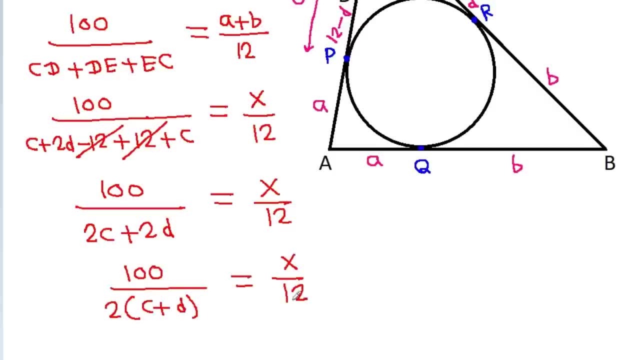 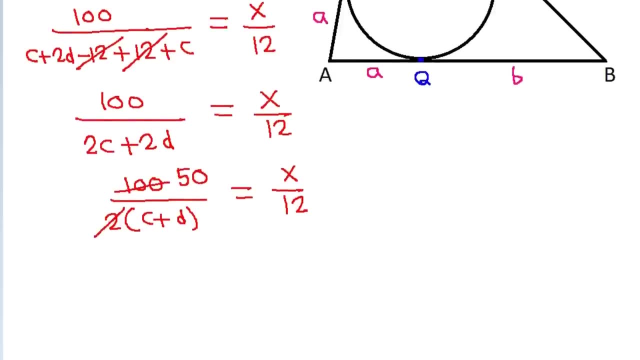 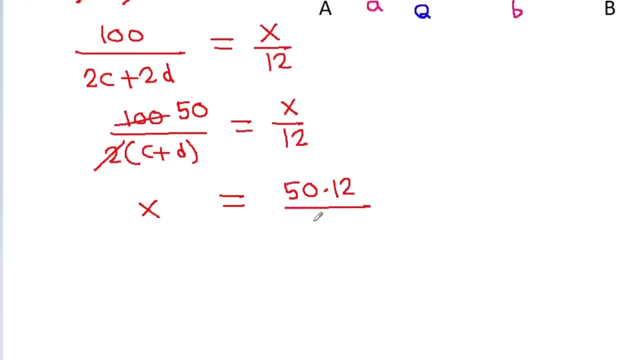 Z And C plus D is equal to X by dual And it is 100 by two times. So nothing is been cancelled. and C plus C 2 times 50 is 100. So x will be equal to 50 times 12 by c plus d, So x is equal to. 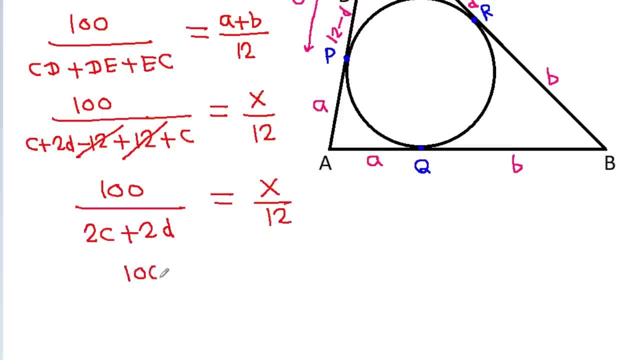 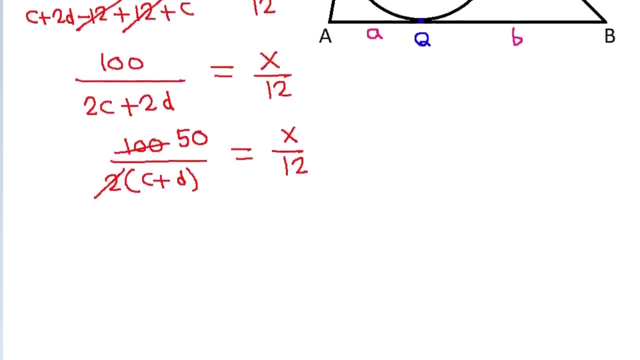 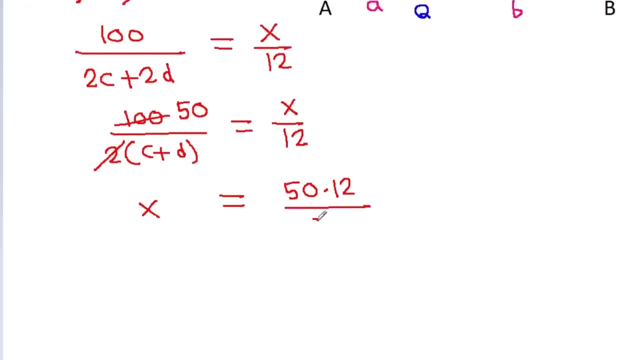 X by 12. And it is 100 by 2 times C plus D is equal to X by 12. And 2 times 50 is 100. So X will be equal to 50 times 12 by C plus D. So 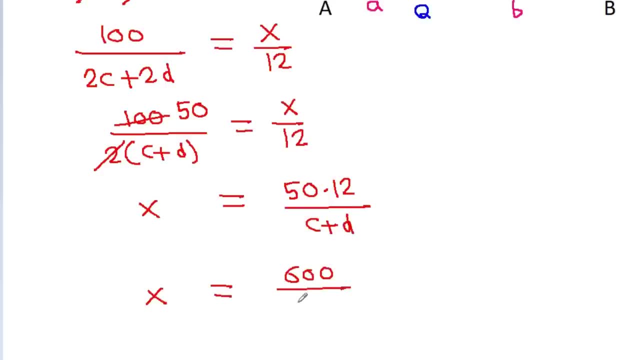 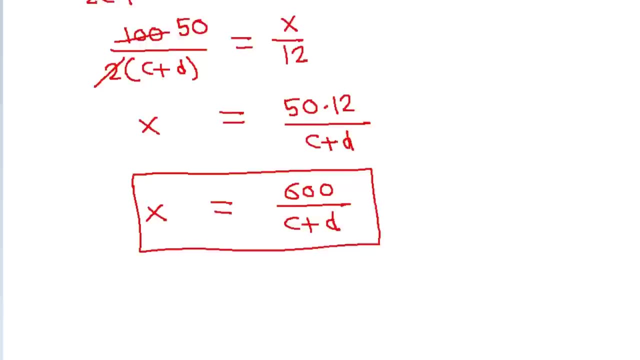 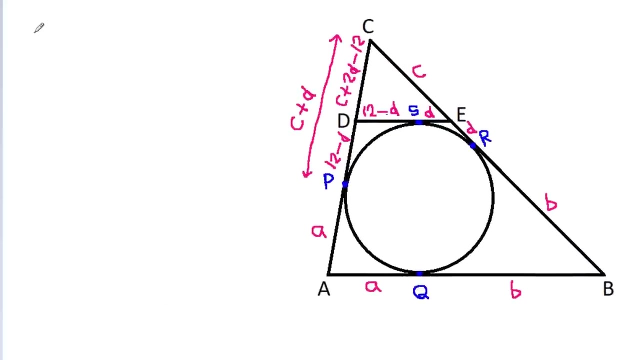 X is equal to 600 by C plus D And we have perimeter of ABC is equal to 100.. And perimeter of ABC it will be A plus A plus B, plus B plus C, plus D, plus C plus D, C plus D, D, It is 100. 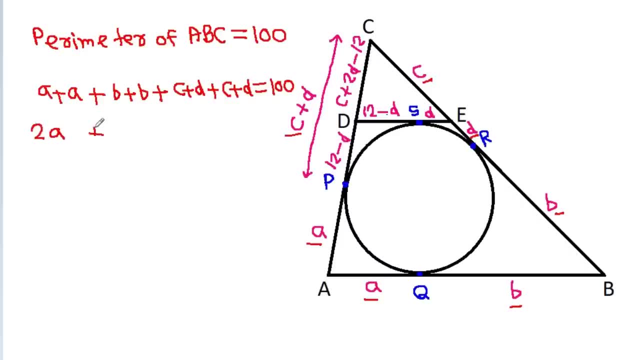 And it is 2A plus 2B plus 2C plus 2D is equal to 100.. And it is 2 times A plus B, plus C plus D is equal to 100.. And 2 times 50 is 100.. 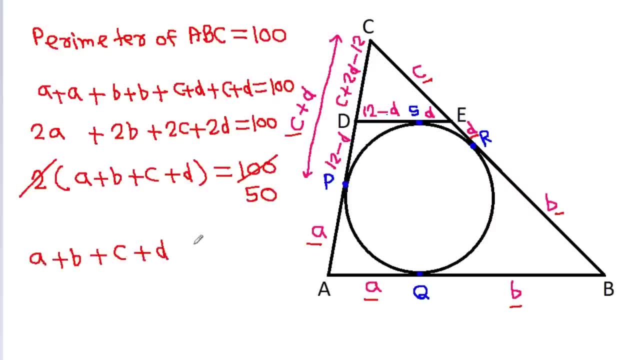 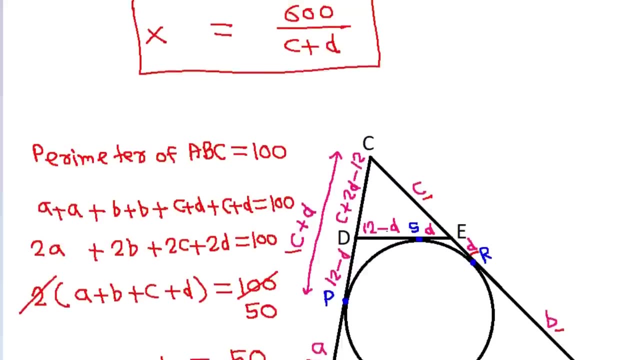 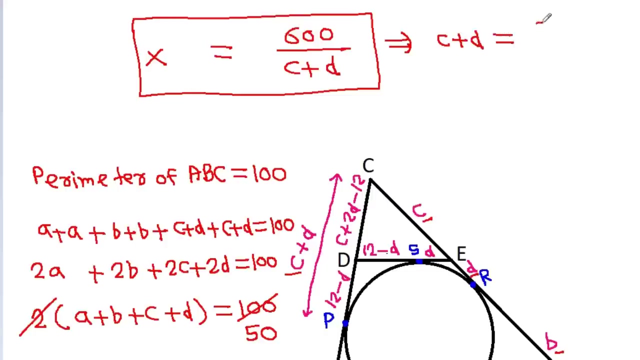 So A plus B plus C plus D, it is equal to 50. And A plus B is X, plus C plus D, it is equal to 50. And from here we can get: C plus D is equal to 600 by X. 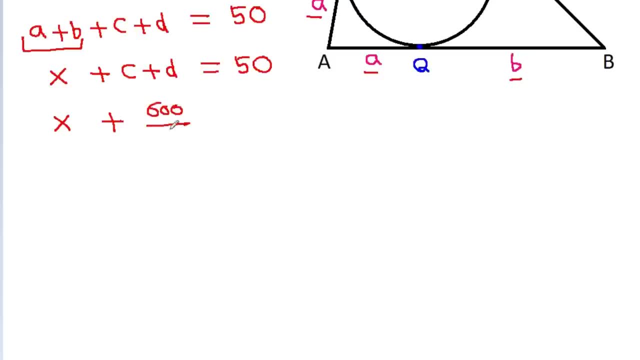 So X plus 600 by X, it is equal to 50. And it is X squared plus 600 by X is equal to 50. And if we cross multiply, then X squared plus 600, it will be equal to 50X. 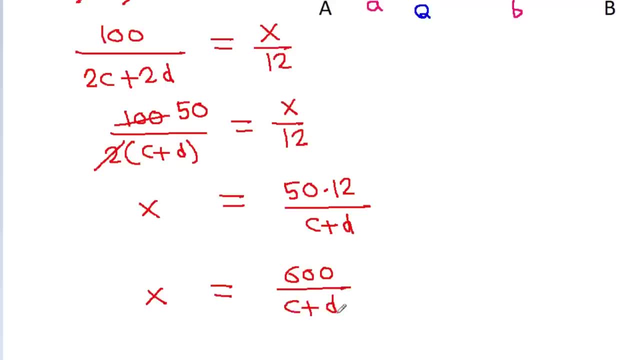 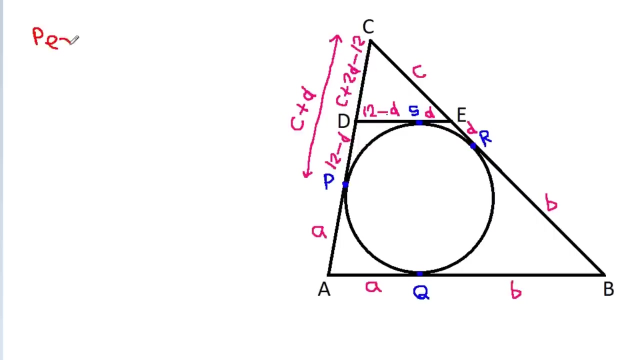 600 by c plus d And we have: perimeter of a b c is equal to 100.. And perimeter of a b c, it will be a plus a plus b plus b plus c plus d plus c plus d c plus d. 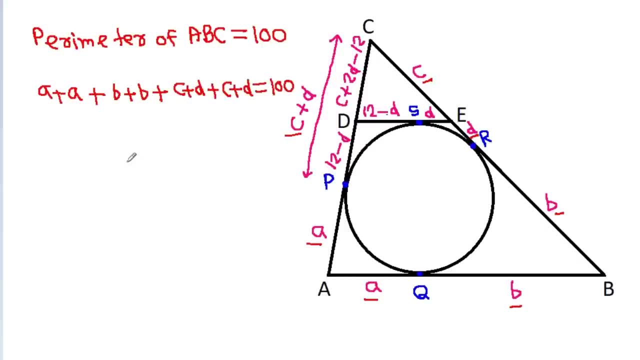 plus c plus d It is 100. And it is 2a plus 2b plus 2c plus 2d is equal to 100.. And it is 2 times a plus b, plus c plus d is equal to 100. And 2 times 50 is. 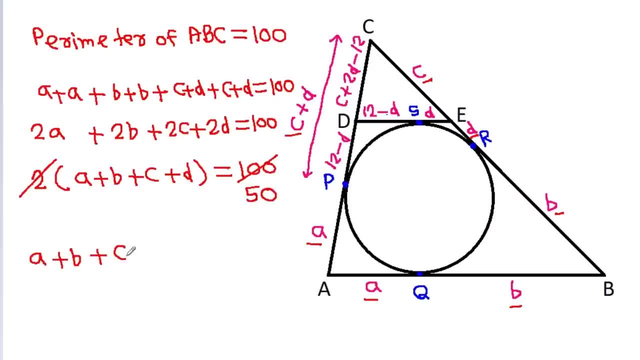 100.. So a plus b plus c plus d, it is equal to 50.. And a plus b is x, plus c plus d, it is equal to 100.. And it is 2 times a plus b plus c plus d, it is equal to 100. And it: 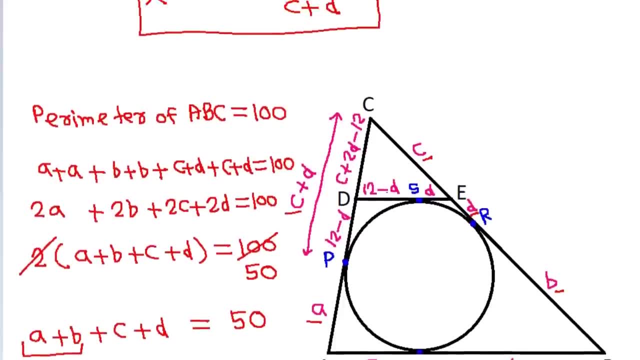 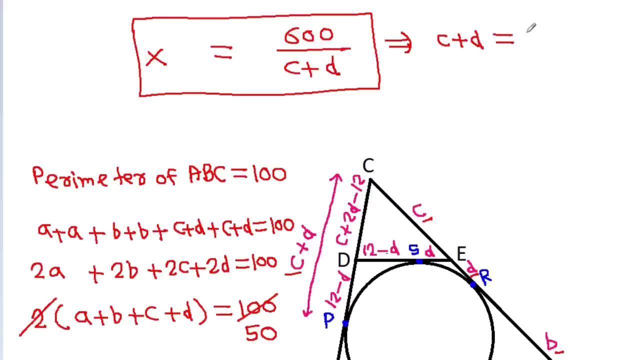 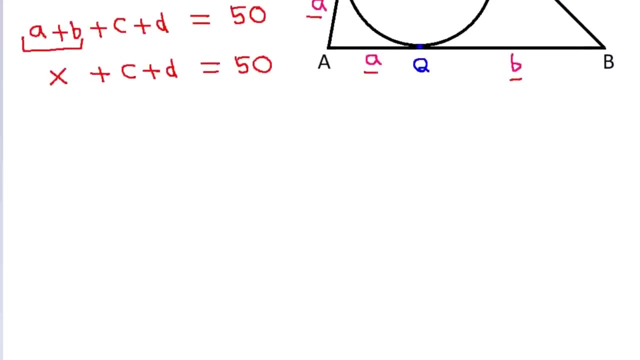 equal to 50. And from here we can get: C plus D is equal to 600 by X. So X plus 600 by X it is equal to 50. And it is X square plus 600 by X is equal to 50. And if we cross multiply, 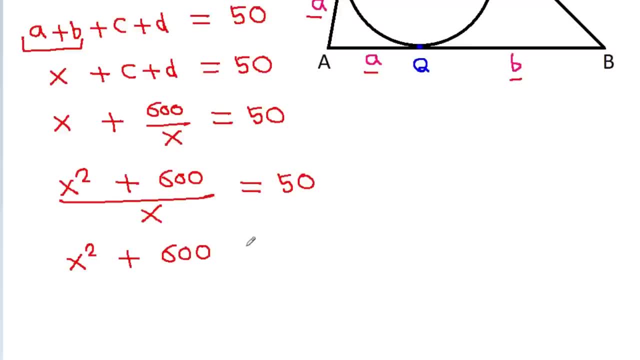 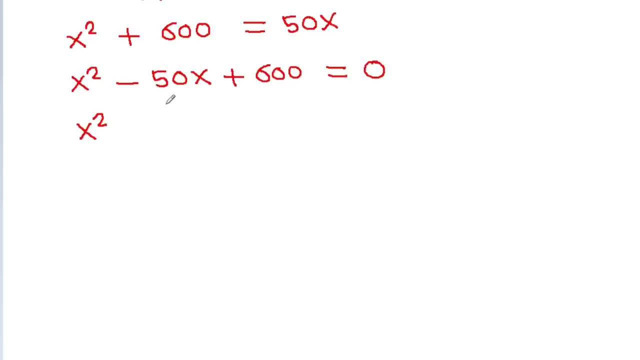 then X square plus 600, it will be equal to 50 X. And it is X square minus 50 X, it will be equal to 50.. So that is 50 X plus 600, it is equal to 0.. And X square and minus 50.